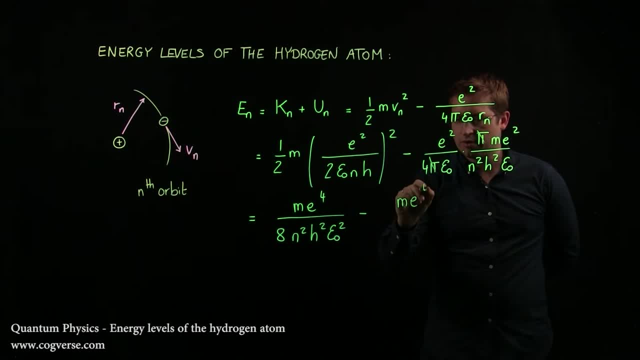 go away. mE squared E. squared E to the fourth, E to the fourth divided by four minus mE to the fourth divided by four. n squared h. squared E to the fourth, E to the fourth, divided by four. 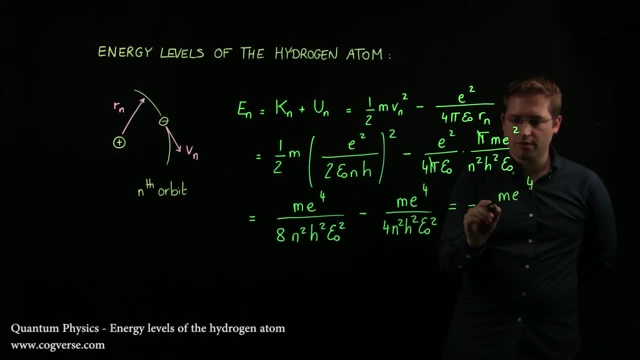 epsilon naught squared, And that is equal to minus mE to the fourth, divided by eight: n squared, h squared, epsilon Not squared. And this is the formula for the energy levels of the hydrogen N squared epsilon, ключ vous Ok. 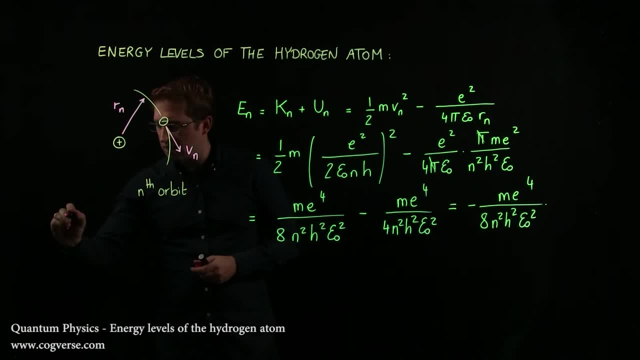 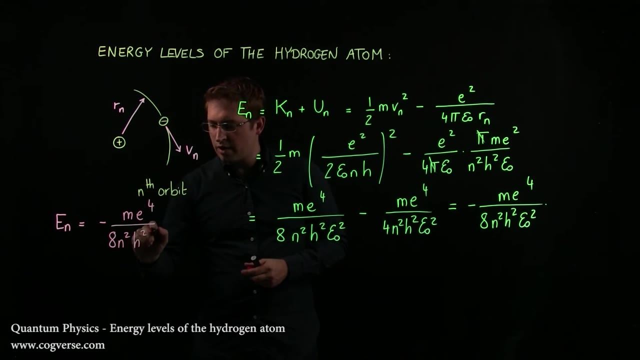 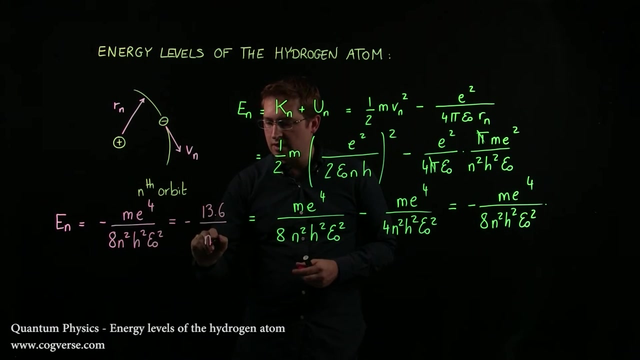 of the hydrogen A squared Persona D, tego 2i2p, an atom E sub n, is going to be equal to minus m e to the fourth, divided by 8. n squared, h squared, epsilon not squared, and that is in fact equal to minus 13.6 divided by n squared. Be careful. 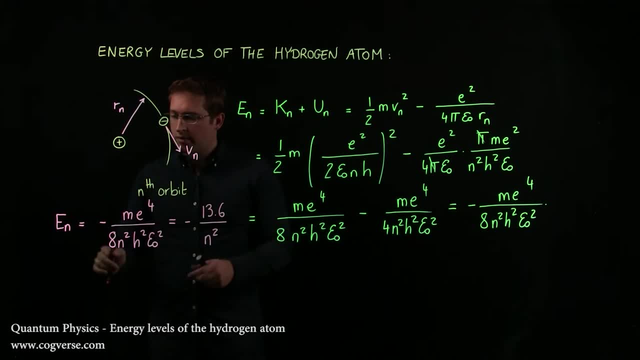 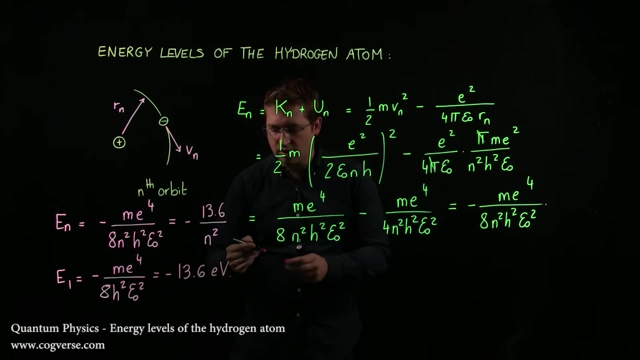 it has to be in electron volts And the ground state has an energy E1 for n equal 1, that is equal to minus m, e to the fourth, 8 h squared, epsilon not squared, and that's minus 13.6 electron volt. 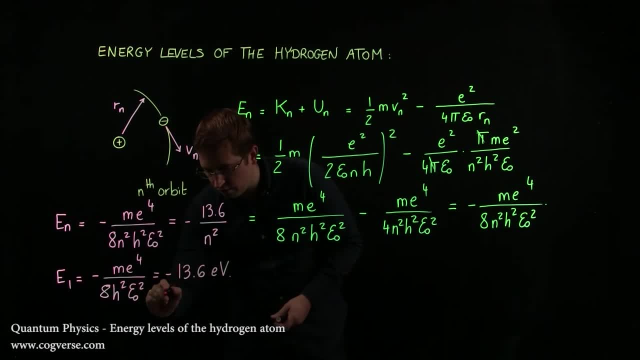 And that, in fact, is the ionization energy. It is the energy required to ionize the hydrogen atom, that is, to rip off its sole electron. and ionization, sorry energy. And that's because it's the energy of the lowest level. So if you 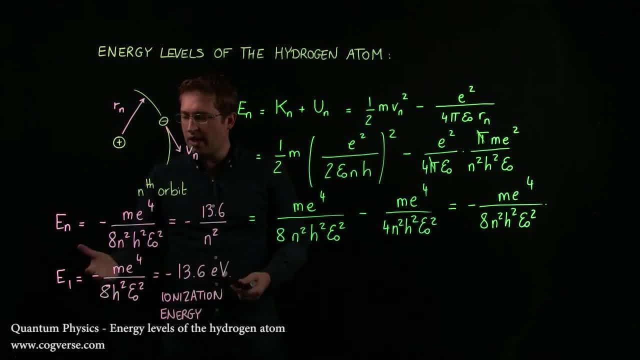 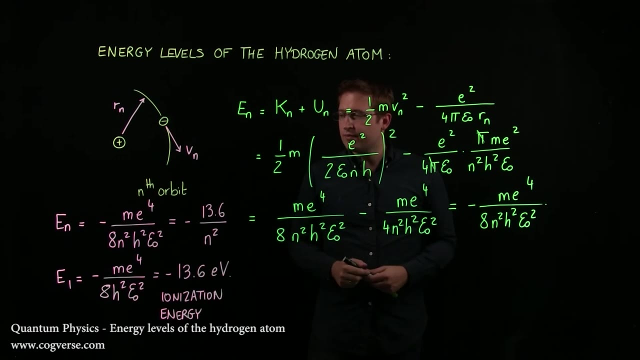 provide that amount of energy, you strip the electron away from the hydrogen atom. Having said that, let's remember that we actually derived a formula previously that was from Balmer's formula and a formula for EN, the energy levels in the hydrogen atom, and we 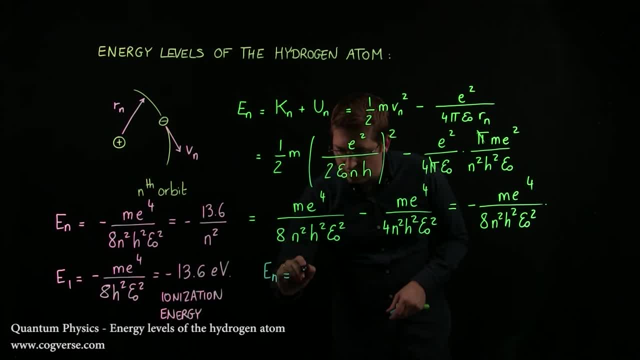 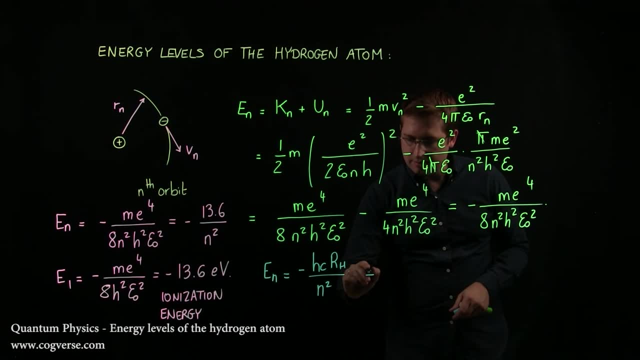 said that we had EN was equal to minus hcrh divided by n squared. Now that implies, if we said this, equal to this, that hcrh is equal toono inhibition of the secretiona n, that is equal to 1.1-squared h.